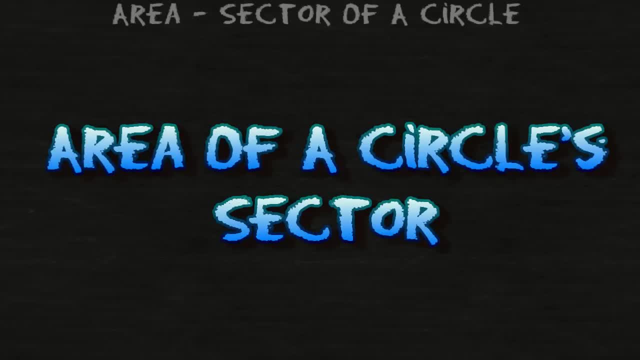 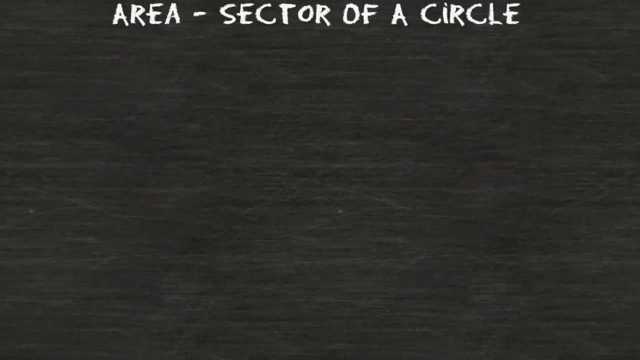 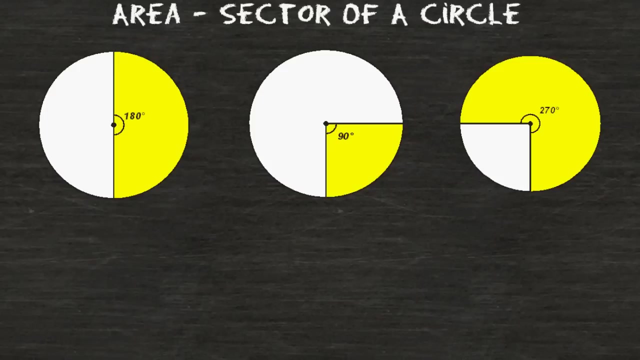 In this tutorial, we are going to demonstrate how to find the area of a circle sector. The first step is to simply identify what fraction of the entire circle is shaded and then multiply that by the entire area of the circle. We already know that the area of a circle is found by multiplying pi times the radius. 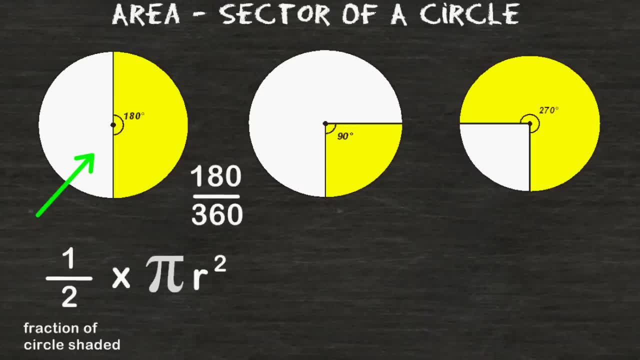 to the second power. Looking at the first circle, we can clearly see that half of that circle is shaded. We can also see that that circle's sector is 180 degrees. So we can say that that sector occupies 180 of the total 360 degrees of that circle. 180 degrees out of 360 is one half. 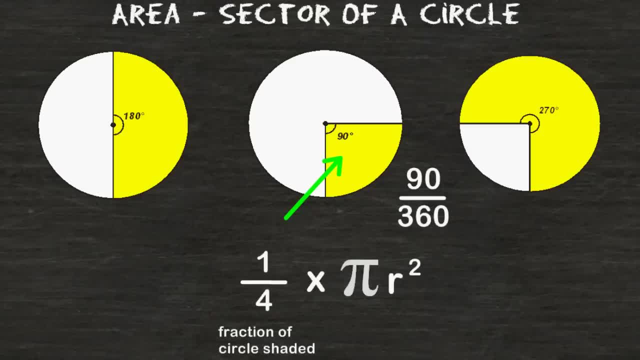 For the second circle, we can see that that sector is 90 degrees, and 90 degrees out of 360 is equivalent to one fourth. So we would multiply one fourth by the area of the entire circle, or take the area of that circle and divide it by four. 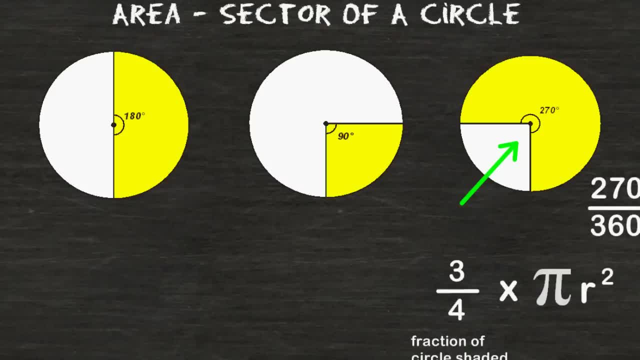 And looking at the third circle, we can see that three quarters of that circle is shaded. so we would multiply three fourths by the entire area of that circle. Also, note that the sector of that circle is 270 degrees, and 270 out of 360 is equivalent. 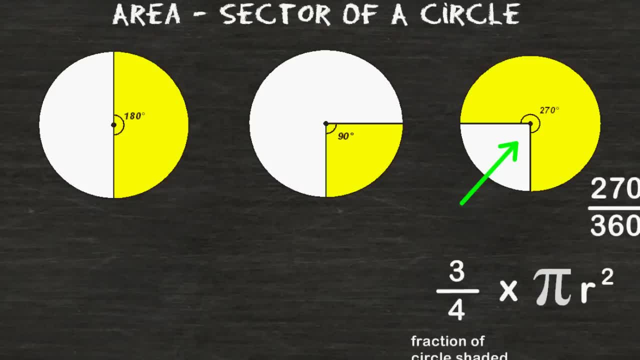 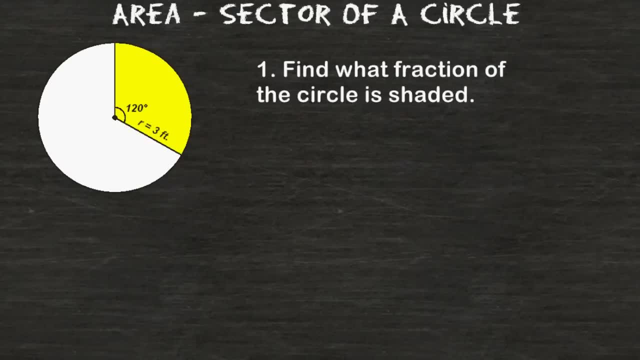 to three fourths. Let's apply what we have learned to an example. First, we are going to identify what fraction of this circle is shaded. We can see that this sector is 120 degrees. 120 degrees out of 360 degrees can be reduced. 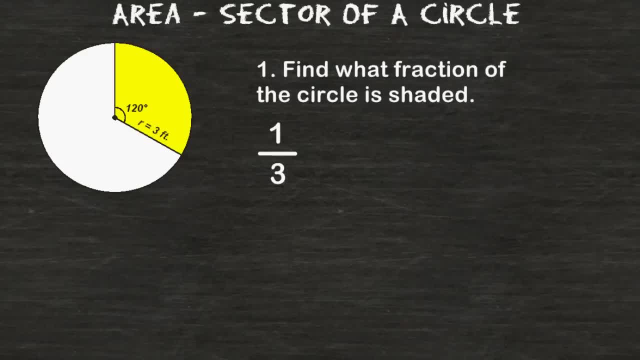 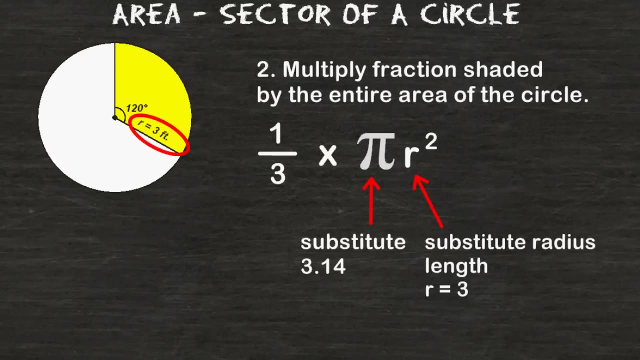 to one third. So in simplest form we can say that the sector occupies one third of the entire circle. So we have to take one third and multiply that by the area of the entire circle. For this example, we are going to use 3.14 for pi. 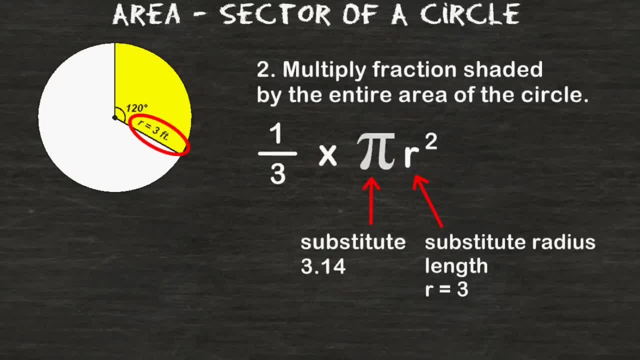 The given radius in this example is 3 feet, so we must substitute the number 3 in for the letter r. After substituting in all of your values. we have to square the radius first, and I am going to simply write that in expanded form.